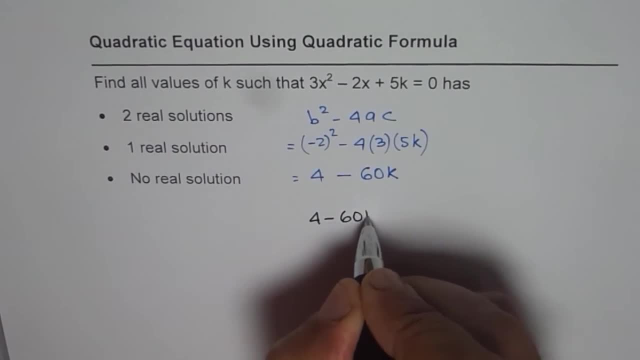 So we'll have 4 minus 60k equals to 0 and we can write this as 4 equals to 60k. So we'll have 4 minus 60k equals to 0 and we can write this as 4 equals to 60k. 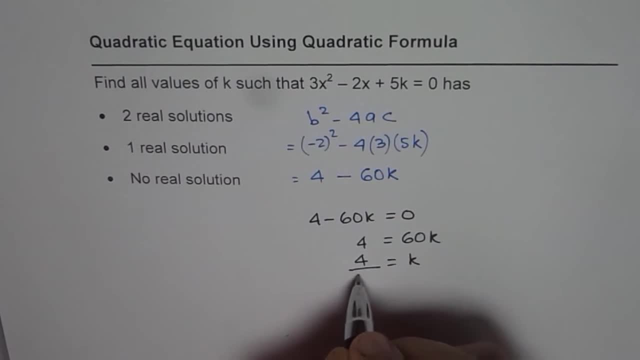 So, for k is equals to 4 divided by 60, right, So this can be simplified a bit, So we can write this as k equals to 1 over, I've got to divide 15, right? So that is what it is. 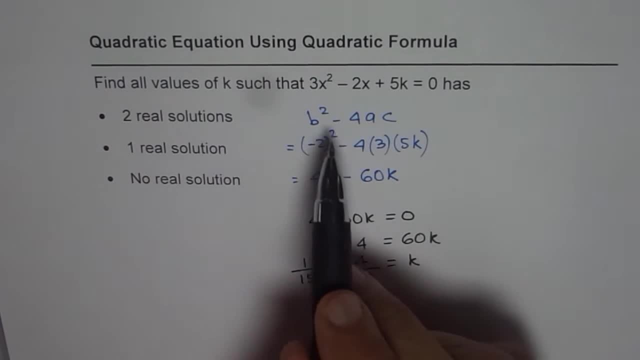 So if k equals to 1 over 15, then b square minus 4ac is 0,. correct, That is what it is. So for k equals to 1 over 15, then b square minus 4ac is 0, correct, That is what it is. 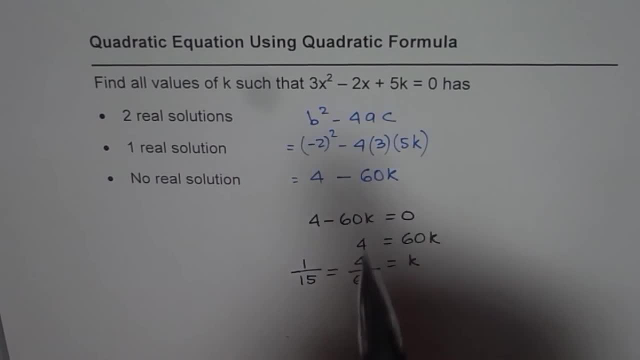 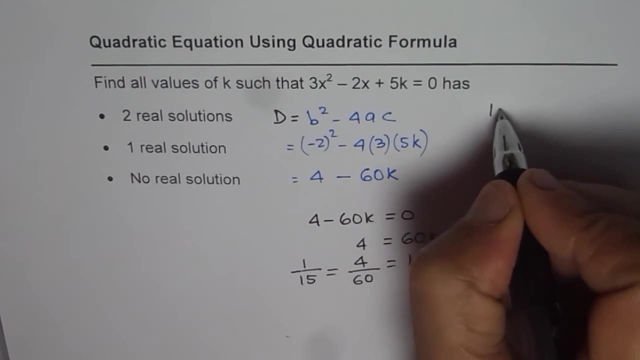 So for k equals to 1 over 15, we have one solution, correct. So let me call this as discriminant. So this is discriminant d, and if k equals to 1 over 15, then d is equals to 0.. 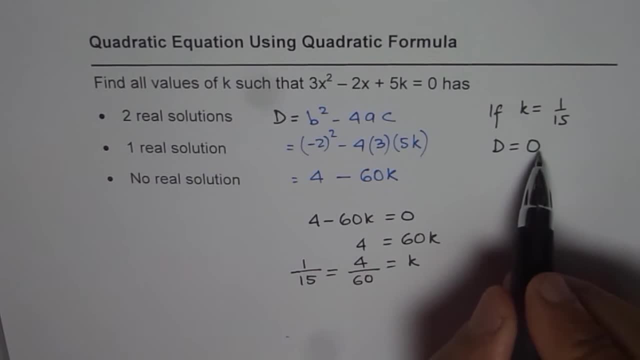 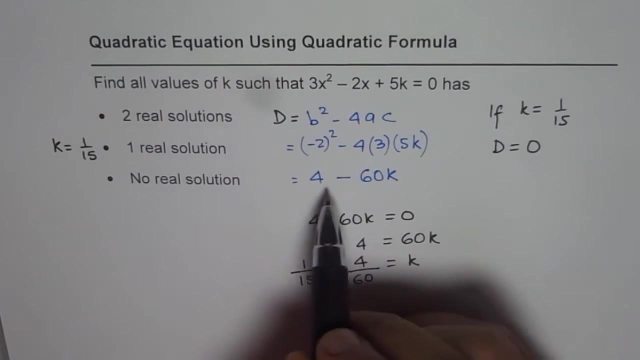 So that means what That means. one real solution, correct? So for one real solution, we have: k equals to 1 over 15, right Now we have to see if k is greater than 1 over 15, then whether discriminant will be positive or negative. That is what you should figure out, right. 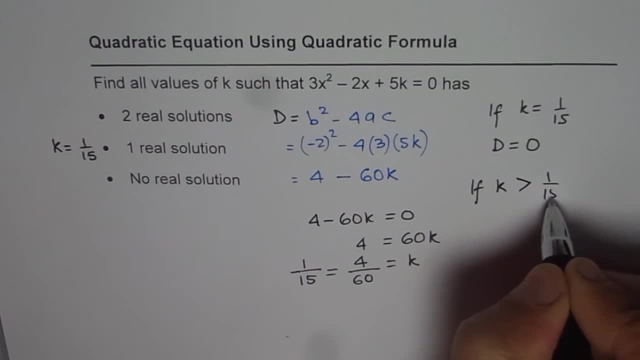 If k is greater than 1 over 15, in that case minus 60k will be greater right. So in that case the discriminant will be negative- will be less than 0, right. So for k greater than 1 over 15, discriminant will be less. 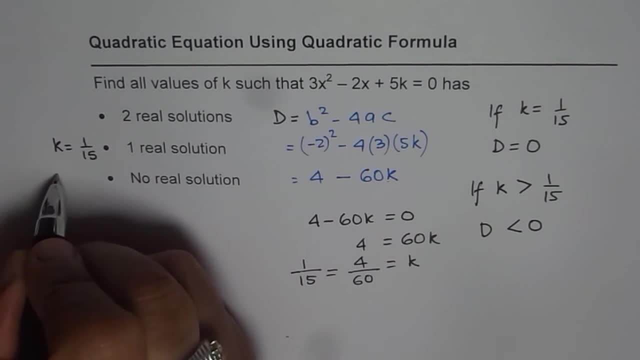 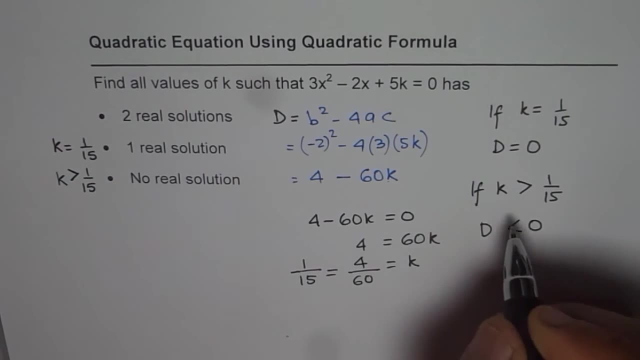 Then 0 means no real solution. So no real solution for k greater than 1 over 15.. Do you see that? And if k is less than 1 over 15, in that case 4 minus 60k will be positive right, Will be positive correct, And so we will have more solutions. 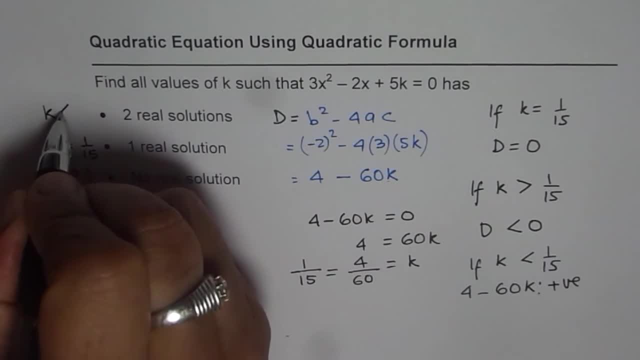 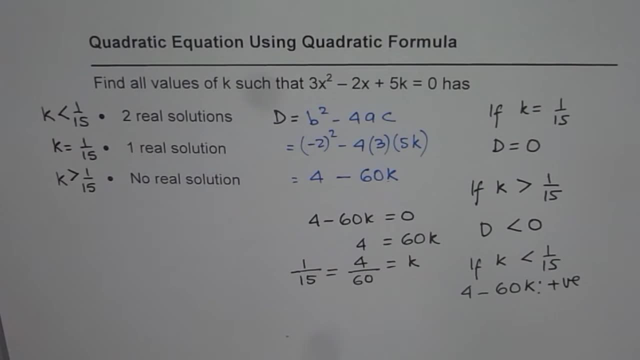 So we will have more solutions, correct. So we will have two real solutions. So for k less than 1 over 15, we will have two real solutions, right. So to summarize, in such a question, what should we find?